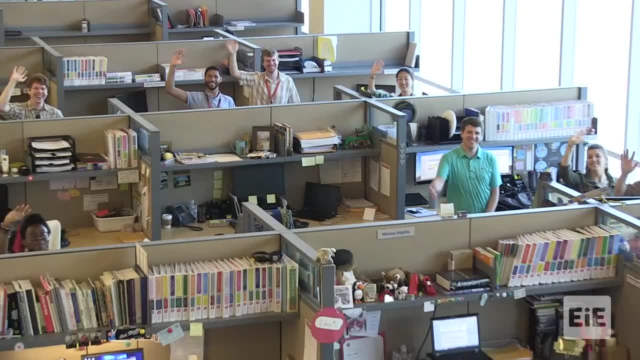 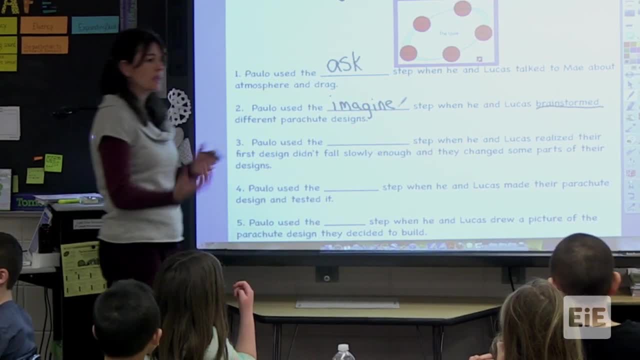 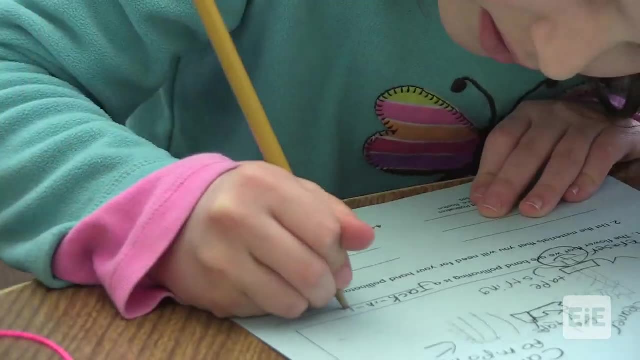 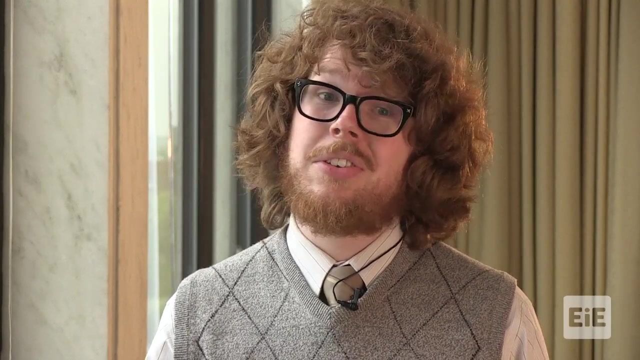 the engineering design process At Engineering is Elementary. we've developed a simplified five-step version of this process that children can easily learn and understand. Encouraging children to use these steps reinforces 21st century skills like critical thinking, teamwork and creativity. The best way to understand the engineering design process is to see it in action. 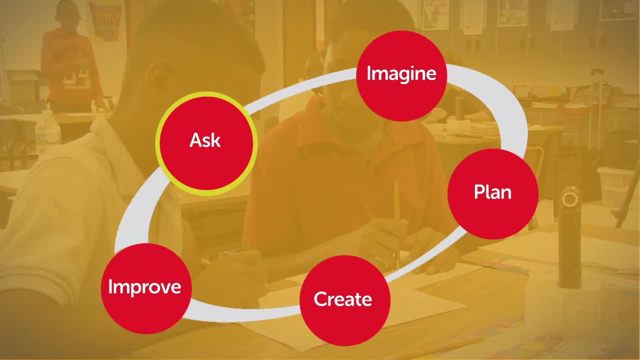 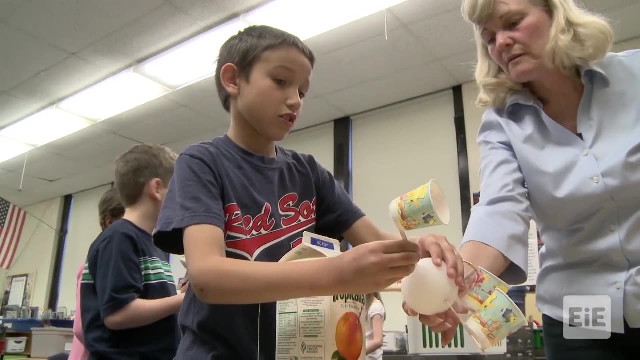 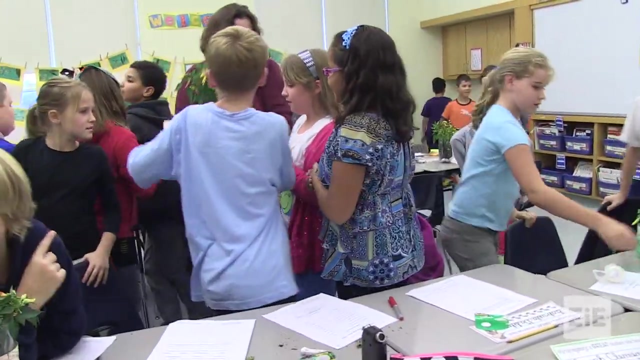 In this video, we will watch children as they ask, imagine, plan, create and improve solutions to engineering design challenges. In the process, they will learn valuable problem-solving and thinking skills that they can use in other areas of their lives Before starting any project. 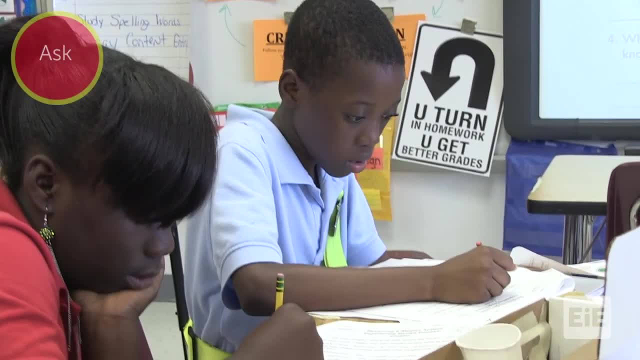 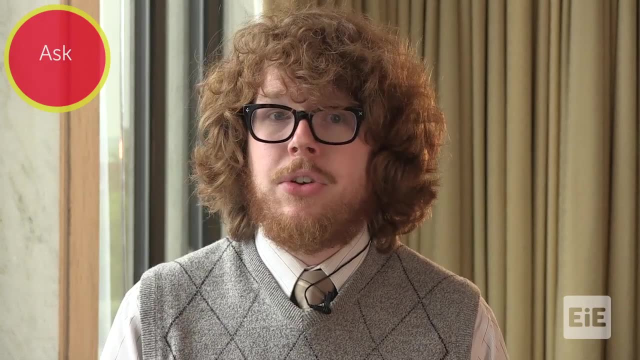 all engineers, children included, must ask and answer questions about the design challenge. During the ask step, children should be encouraged to think about what they need to know in order to solve the problem they're presented with. Some questions might be about the science. 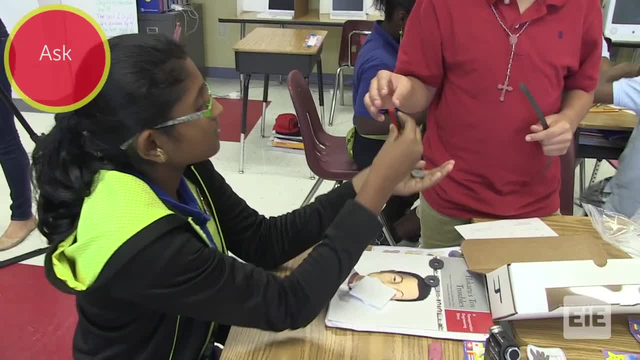 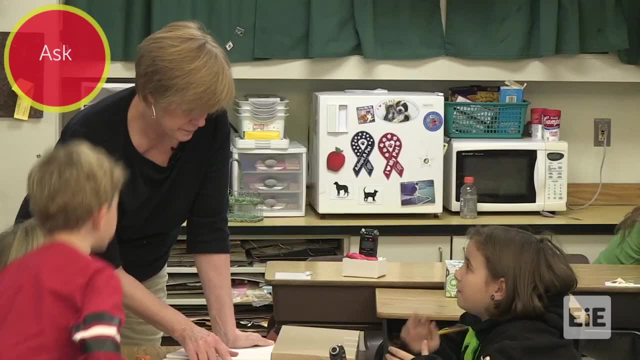 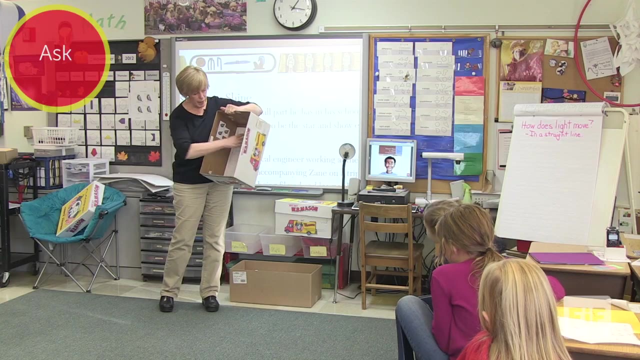 behind the problem. others might be about the specific goals of the technology they're creating, and others might be about the materials that they're going to have to work with. In this clip we see third graders in Fairfax, Vermont, practicing the ask step. Sandy Brown has introduced her students to a design challenge. 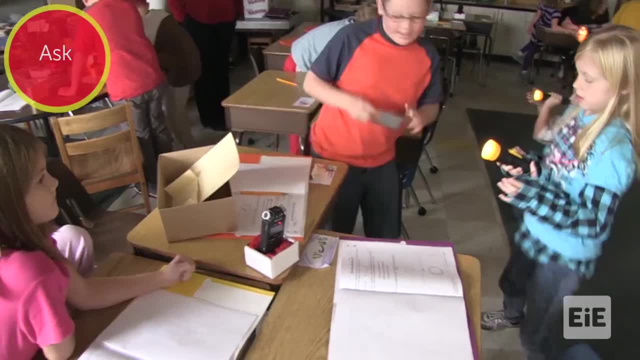 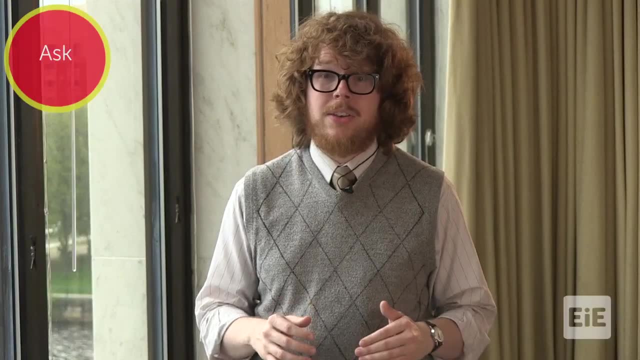 in which they need to use a mirror to reflect the light from a flashlight to different parts on the inside of a box. She challenges her students to think deeply about questions they need to answer in order to produce a successful lighting design. Now you get to ask me questions. 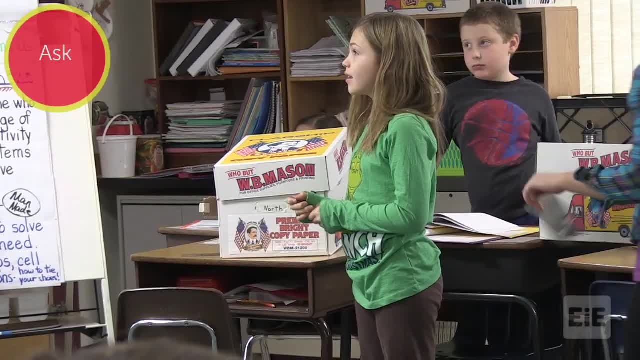 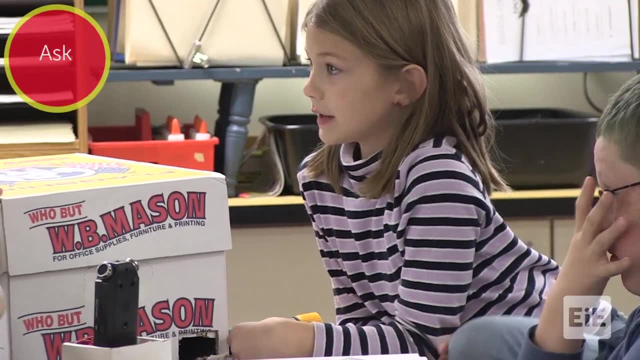 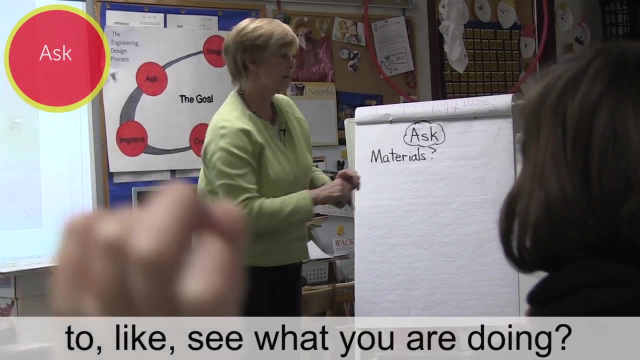 We're going to be in the ask stage right now. What do you want to know about this project, Lexi? What kinds of materials? What types of materials are we using? What type of materials Do you get different light sources to see what you're doing? 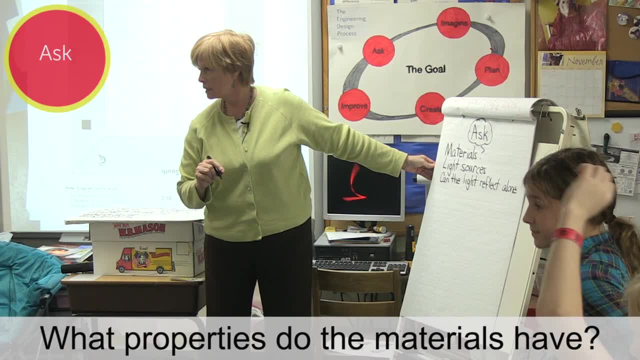 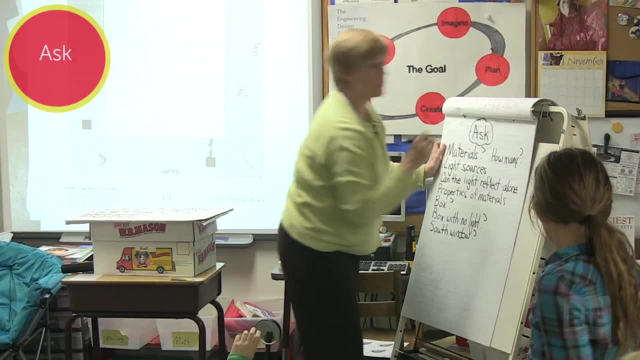 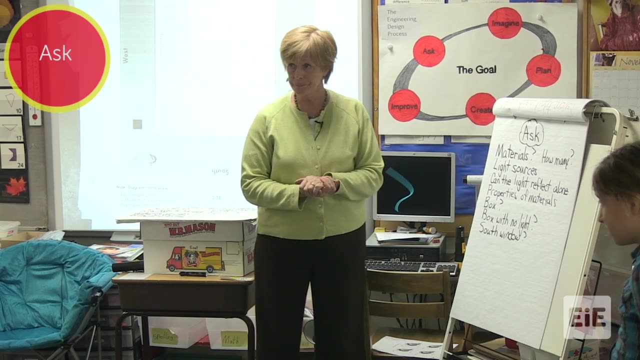 Yes, What properties do the materials have? Oh, that's a good question. So I'm going to stop for a minute and what I'm going to do is show you the first one. I'm going to show you the first one. 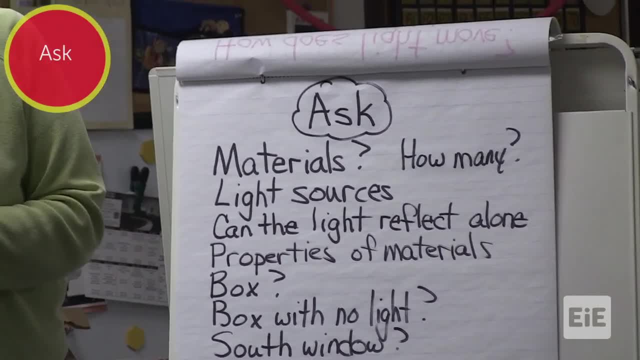 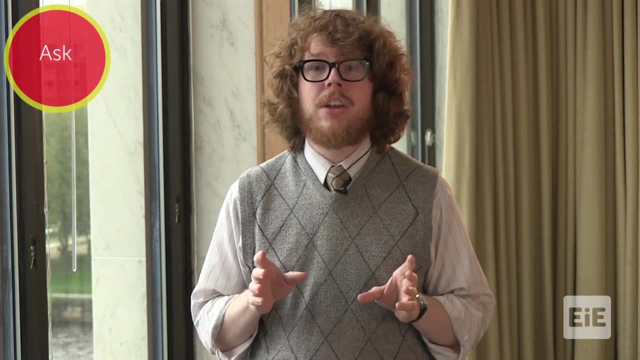 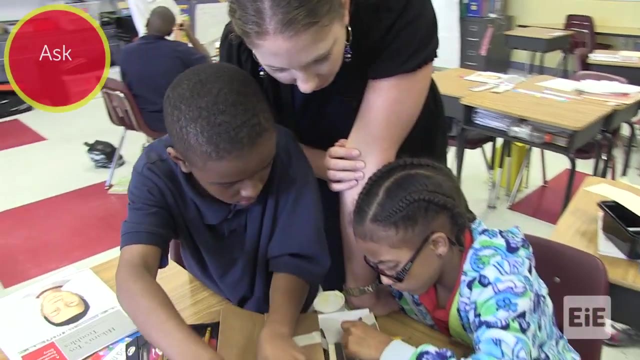 I'm going to show you what materials will be available to you. Asking students what they need to know, rather than telling them, provides an opportunity for students to think critically about what exactly the problem is and how they might start solving it. The ask step helps them to begin to identify as problem solvers. 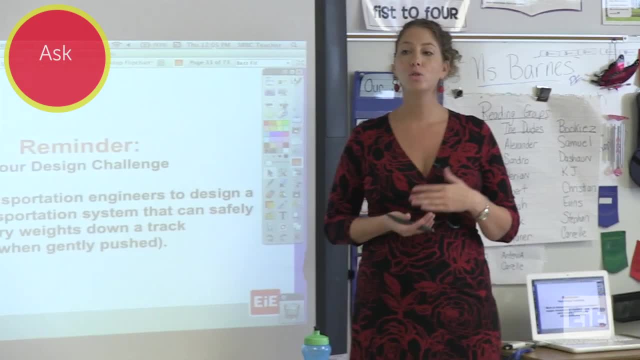 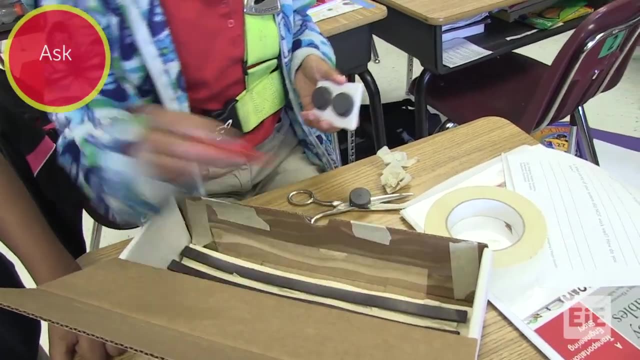 Let's take a look at another class, this time in fifth grade. The teacher, Deborah Kelly Thomas, is having students review what they know about materials and having students review what they know about magnets to prepare for a magnetic vehicle challenge. At this point, Kelly's students have spent several hours on the ask step. 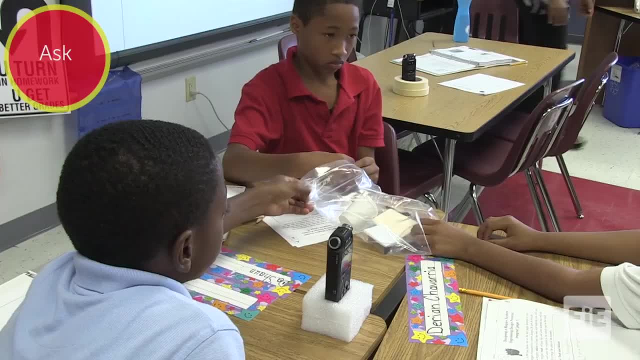 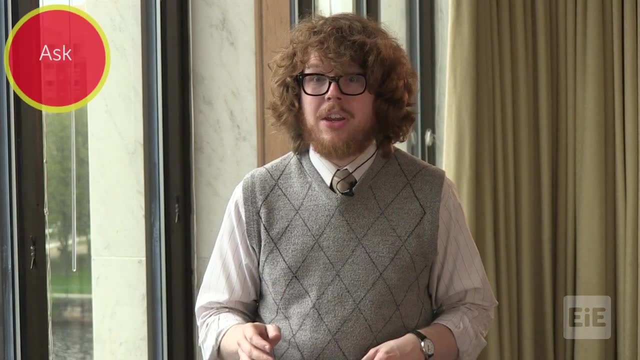 They've explored different types of magnets and how strong they are. They've looked at the materials that they'll have available during the design challenge And they know how their vehicles will be tested for safety and efficiency. Remember, we're still in the ask phase, so I want you to stay on the front sheet. 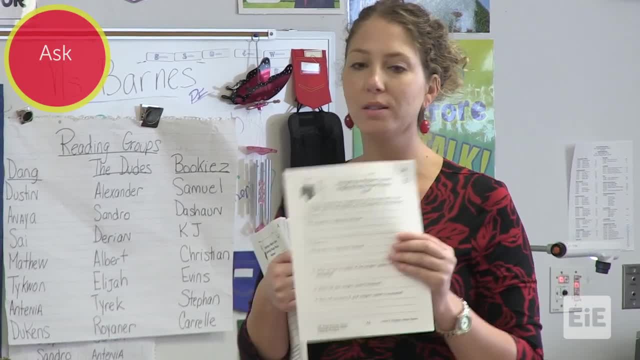 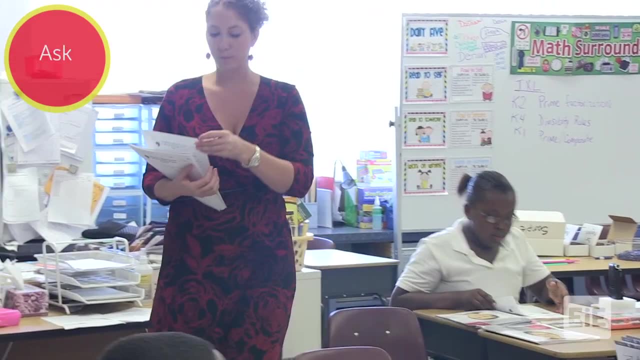 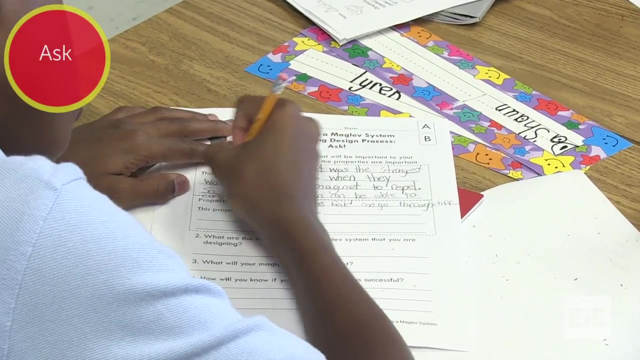 And in the packet it's asking you to list two properties of magnets that we can use. that will help us to design our Maglev package transportation system. Okay, let me share with you what Corelle put. Corelle says: property one: the repelling of the poles. 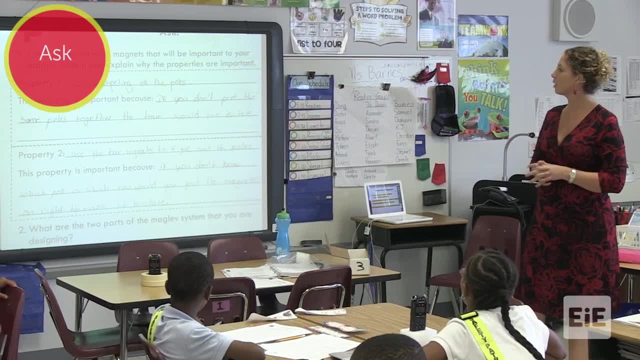 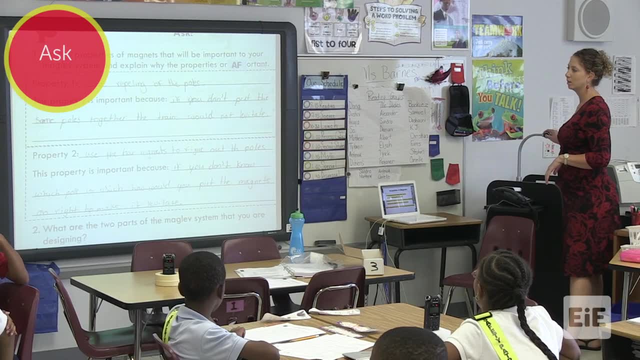 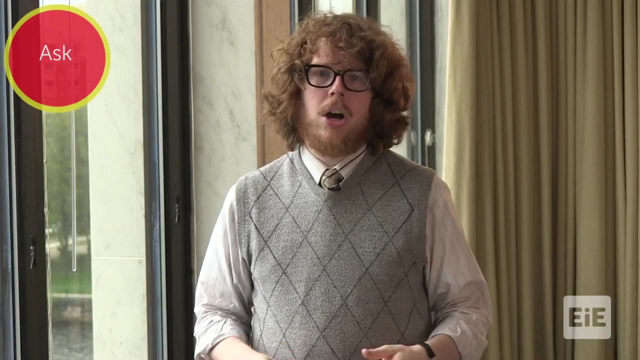 She said this property is important because if you don't put the same poles together, the train would stop. The train would not levitate. Okay, so that's a property of magnets that's going to help her in designing her Maglev system. 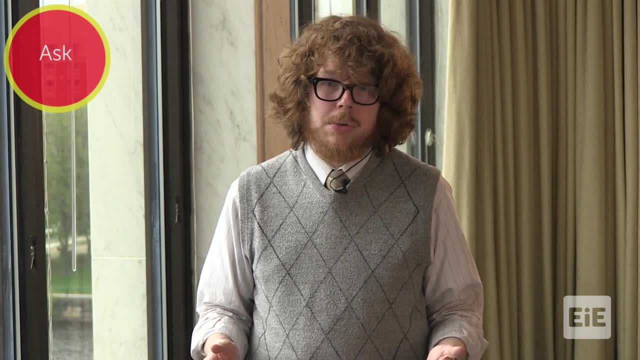 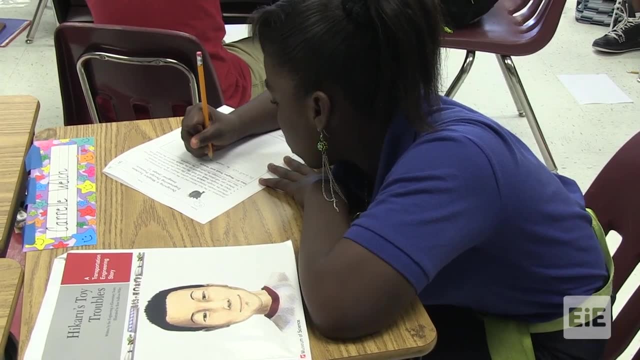 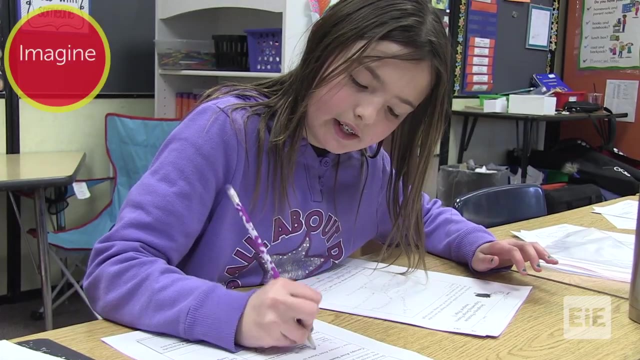 Although students continue to ask and answer questions throughout the unit. this first step provides all learners with the baseline information they need to know to move forward In the second step of the engineering design process. Imagine students start to brainstorm solutions. In this step, the goal is for students. 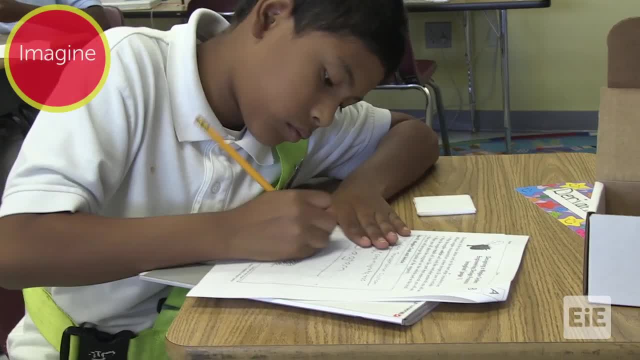 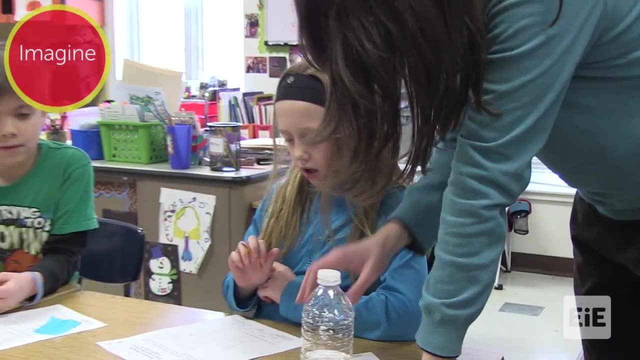 to independently come up with ideas, and they're encouraged to think creatively and without judgment. Individual students may respond differently to this type of challenge. Some students may not be as used to imagining more than one way to solve a problem. For others, 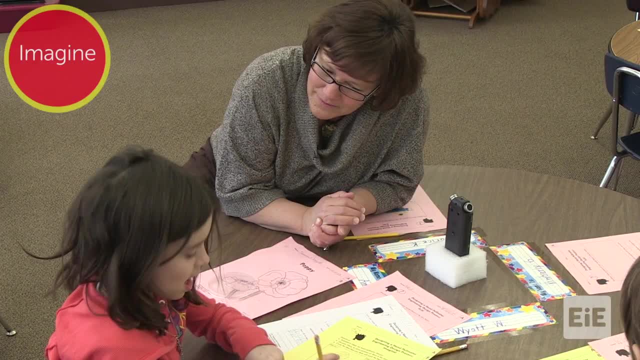 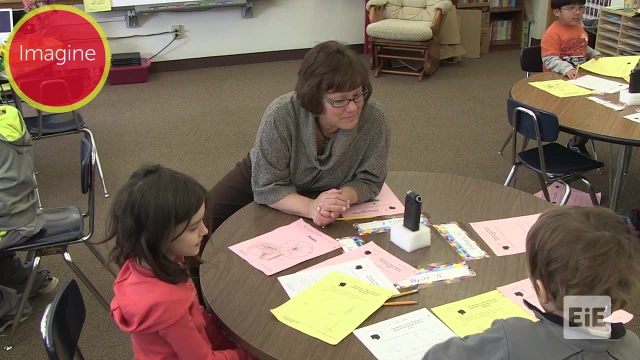 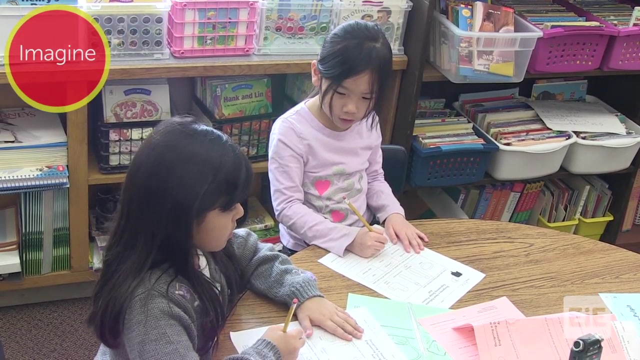 brainstorming multiple possibilities is a true strength As a teacher. it's important to acknowledge both the struggles and the rewards of navigating the Imagine step. In this next clip, first graders are imagining different ways they might move pollen from one plant to another. 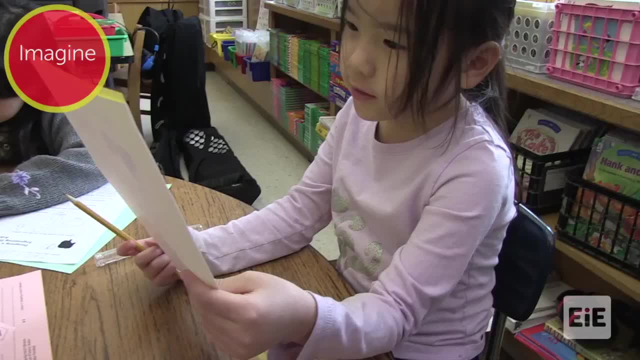 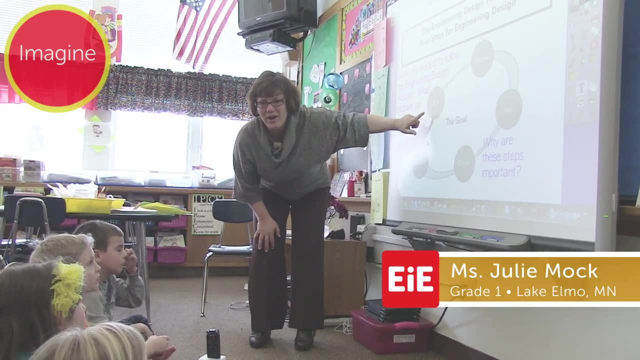 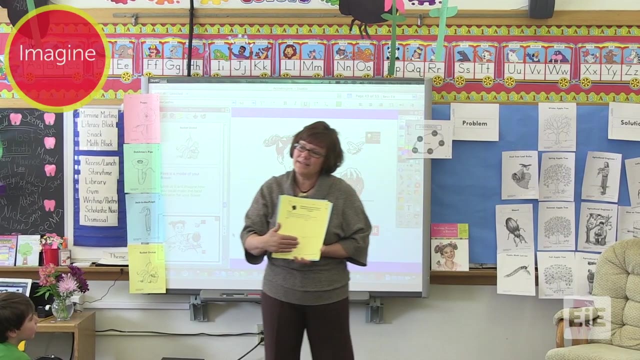 by hand. Their teacher, Julie, explains what she expects of her young students as they go through the Imagine step. If we started with, ask, where are we today? Imagine We need to go to. Imagine We have four different boxes, and you know what I'm hoping for. 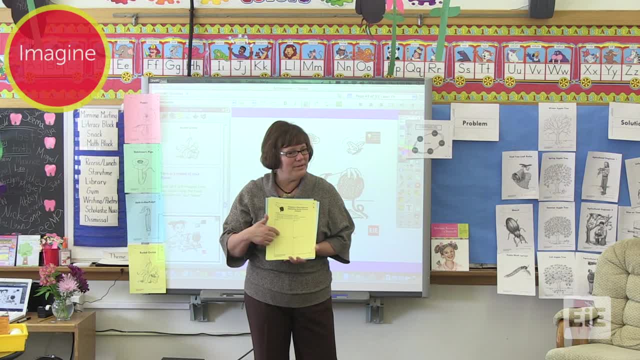 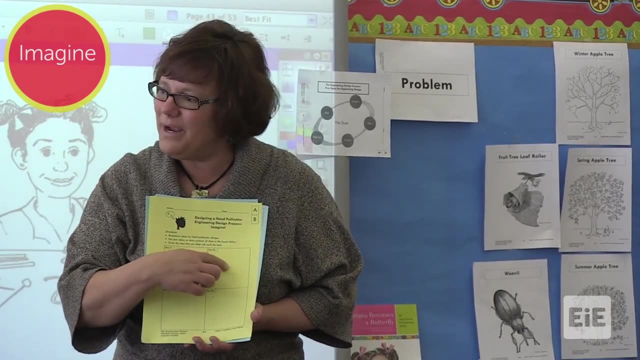 I want you to imagine one way of building a hand pollinator and drawing it right here. Label your pieces, your parts, label it so you know what you planned there. Then think of different materials and a different way to make a hand pollinator for box number two. 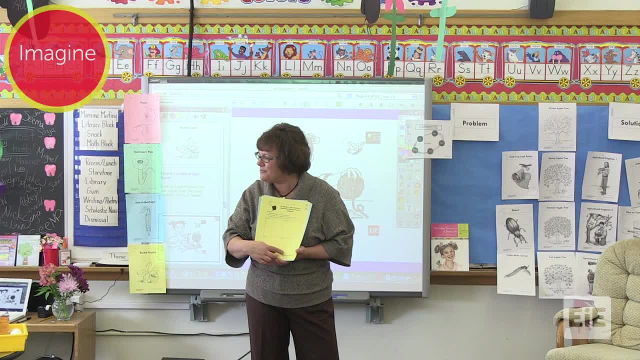 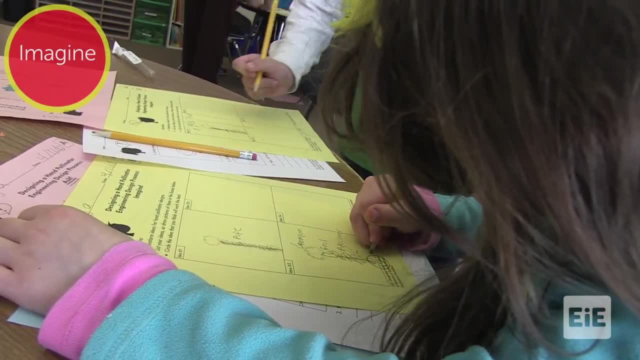 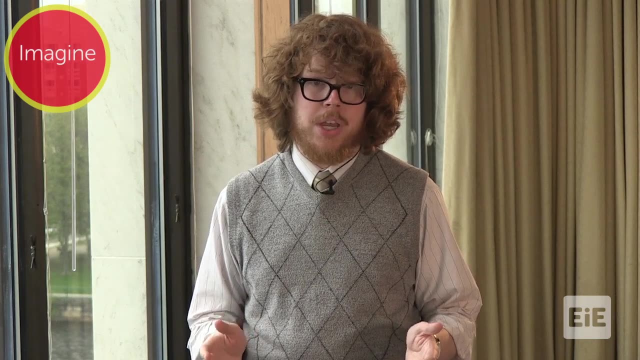 And yet a different one for three and another different one for four. The Imagine step allows students to experience the innovative, creative thinking style that has led to many of the world's engineering breakthroughs. In this next clip, Cory Christensen prepares her third graders. 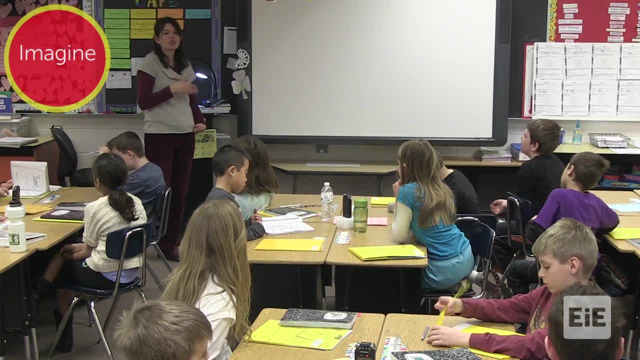 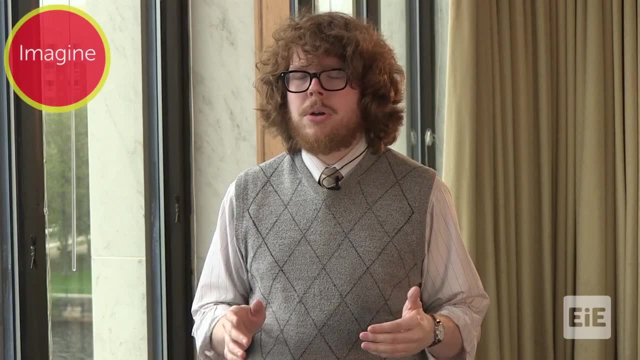 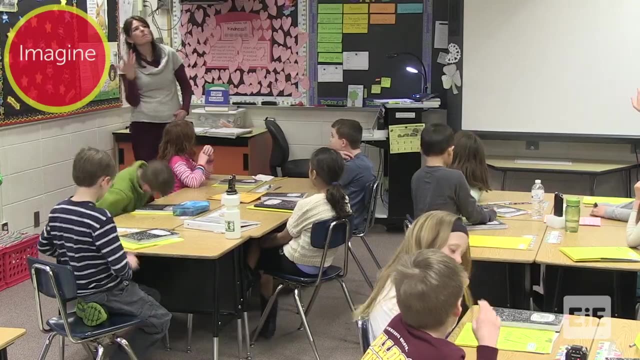 as they start to imagine solutions for an aerospace engineering challenge. They are to design a parachute to land on another planet. Before they brainstorm, Cory provides examples from history to impress upon her students the importance of thinking outside the box. How are some of the 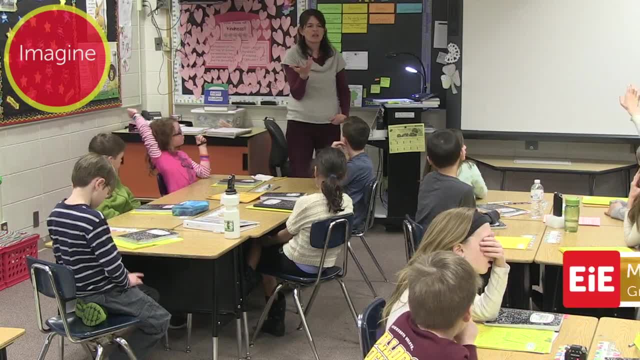 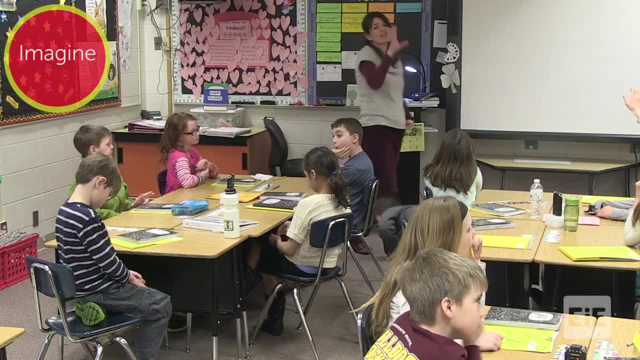 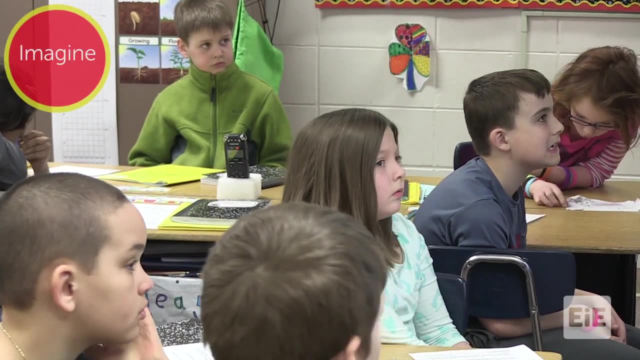 most important inventions created By imagining. By imagining them and just crazy, outrageous ideas that many people said there's no way that could work. Do you think everybody thought a person could go to the moon? No, What do you think that a lot of people 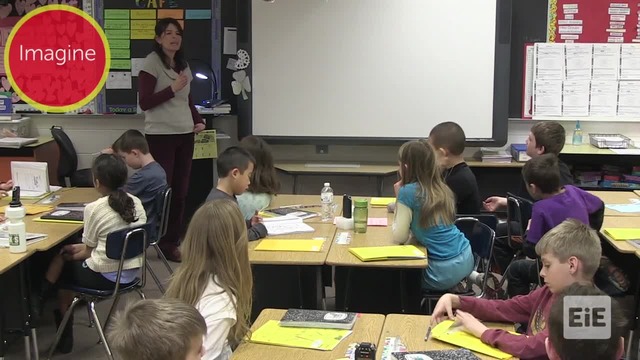 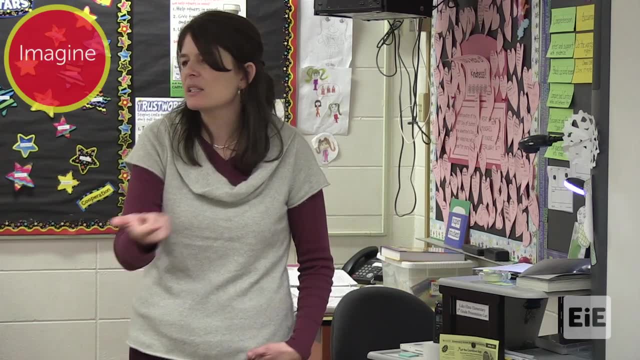 probably told them: You can't do that, It's impossible, It's impossible, You can't do that. And so if they just said, I'm going to be able to go up to space. So there's a lot of different things. 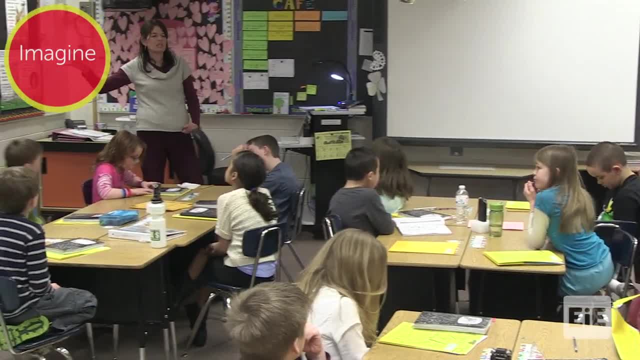 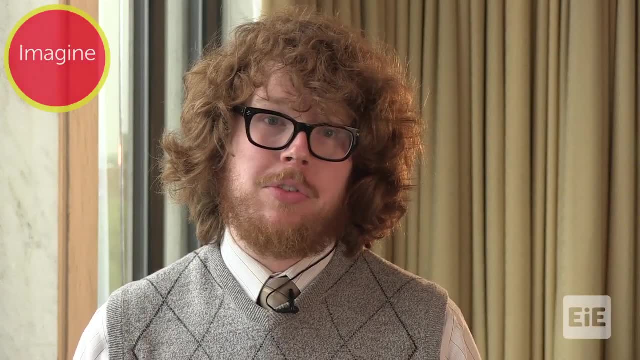 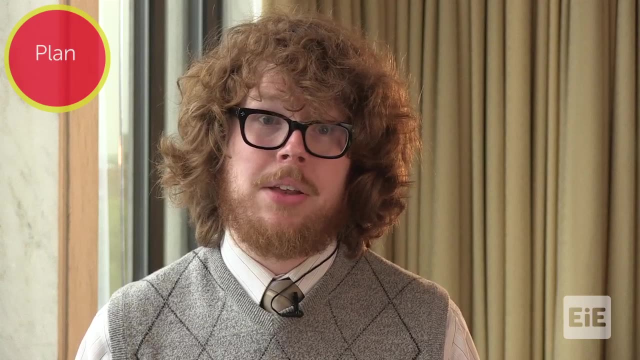 that are there because people do imagine all these possibilities and are brave enough to take that step. The imagine step reinforces that there's more than one way to solve a problem. It prepares students for the next step plan, where they'll focus more deeply. 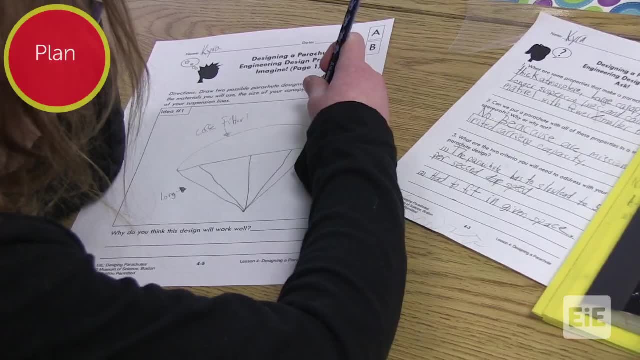 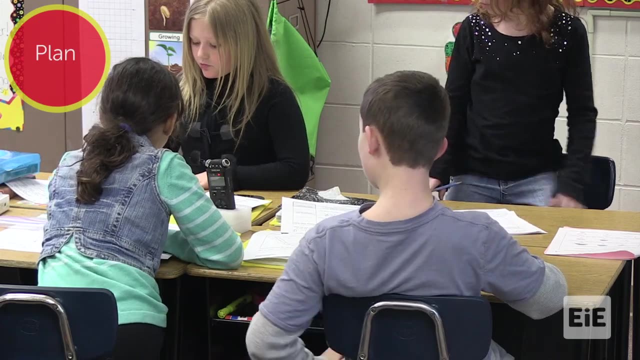 on the one design they want to create. So when you get together, you're going to be combining all of your ideas together. You come up with all these individual imagine ideas. then they come together and they talk about why would it work? why wouldn't it work? 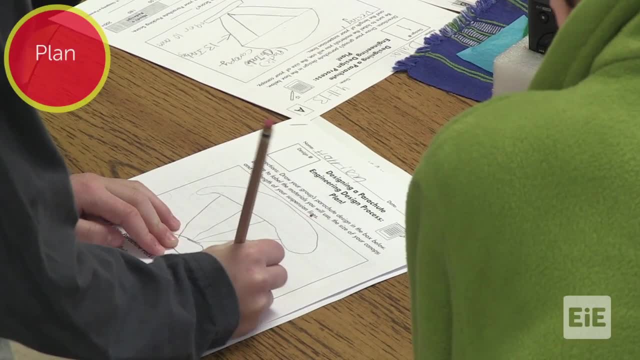 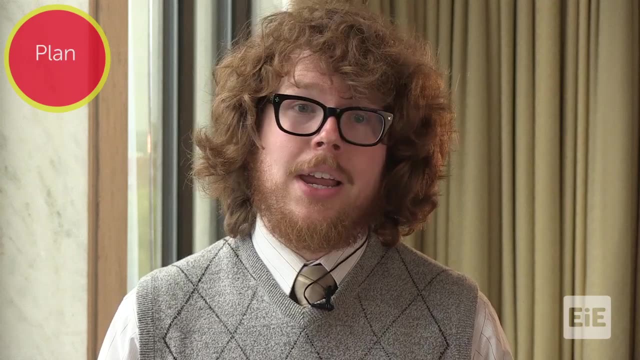 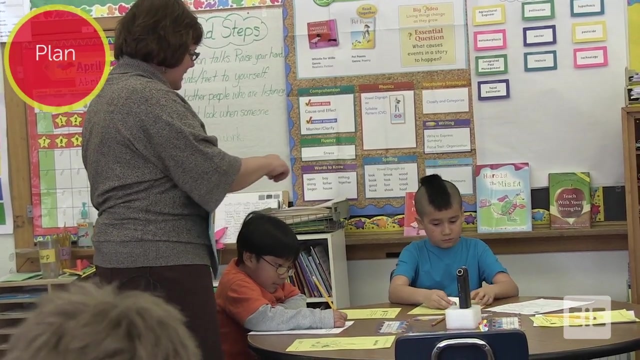 As Corey explained, during the plan step, groups of students must choose one imagine idea that they'll further develop and test Back in first grade. Julie introduces the plan step to her students as they choose designs for hand pollinators. Her comments focus on teamwork. 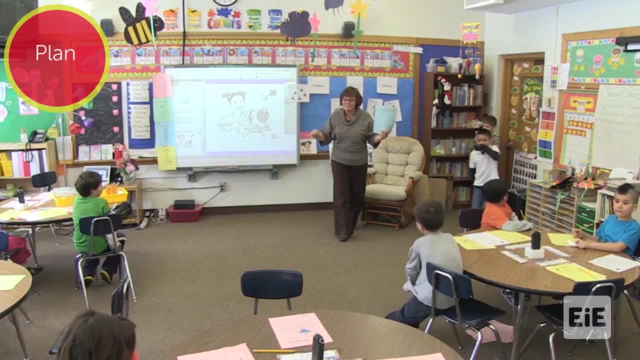 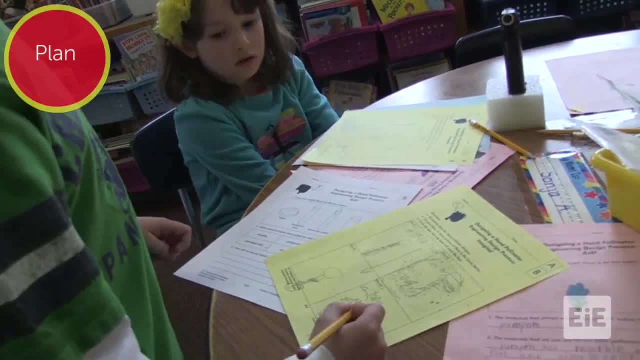 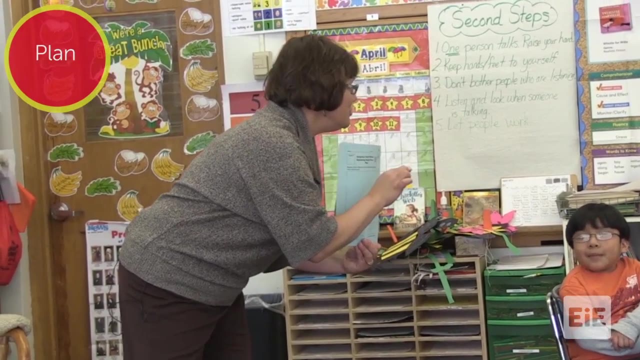 encouraging compromise and collaboration. It's time to make a plan. Draw a diagram on this big box now. Out of all four of those, which one do you like the best? And add labels so we know what materials you're using and how they're connected. 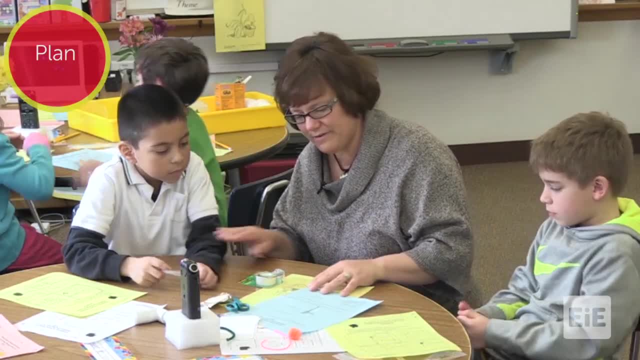 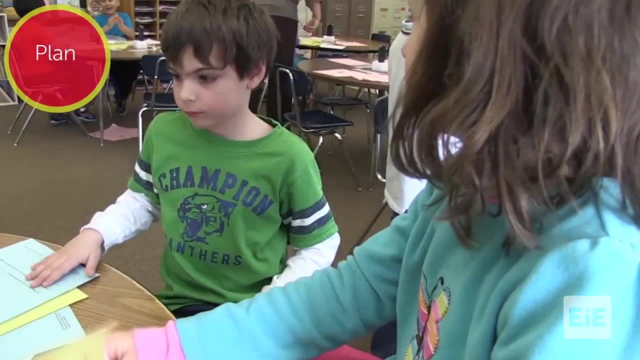 Are you ready? Okay, Tell me what you have here. Do you guys agree on this plan? Do you like it together? Oh, great teamwork. So let's say number three, but we'll just bend number three. How about that? 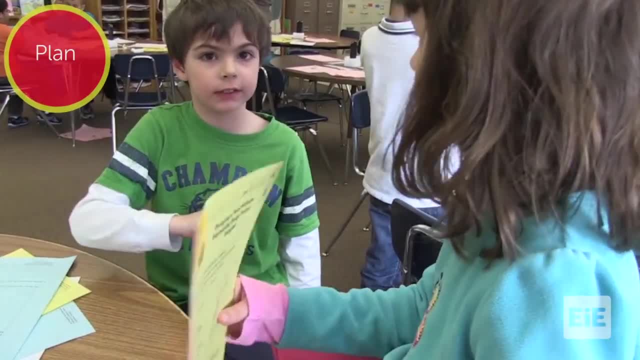 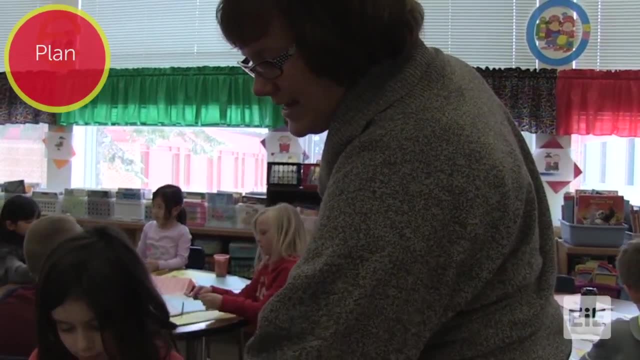 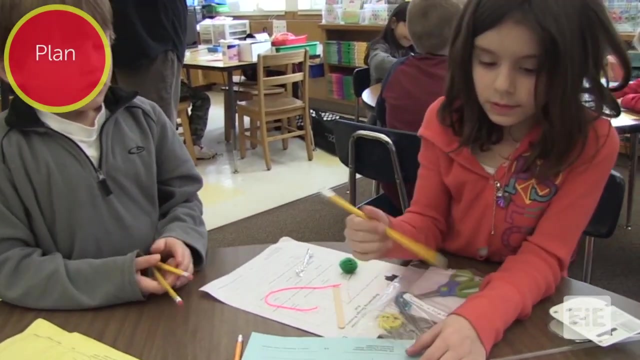 It will look like your idea, but it will do the things that are in my idea. I love how you are writing your supplies and drawing what you think it's going to look like. That is great thinking. I'm loving your cooperation there. 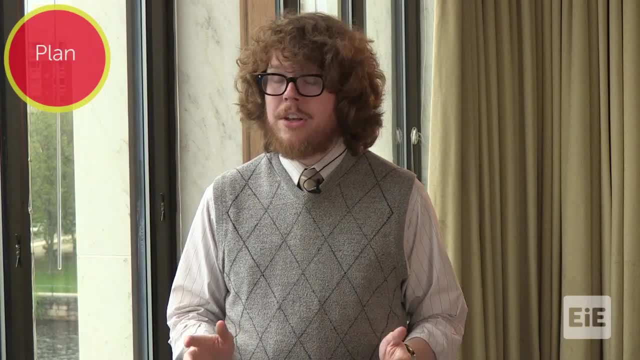 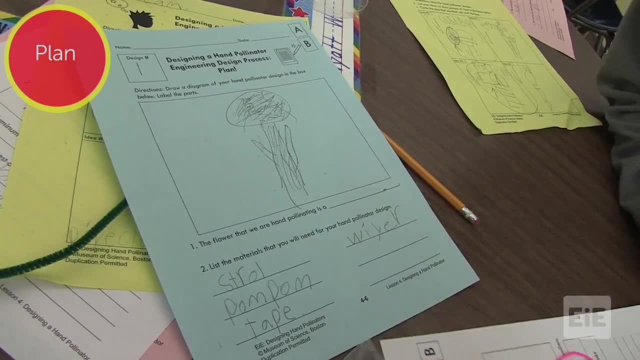 After discussion, the group records their final plan. They know that they're about to actually create this technology, so they're motivated to label their drawings and write down the materials they're going to need Only after students have asked and answered lots of questions. 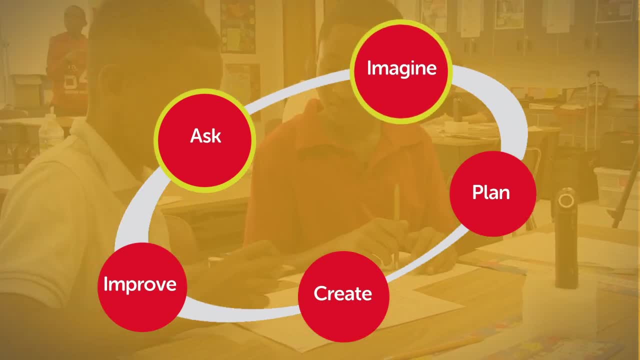 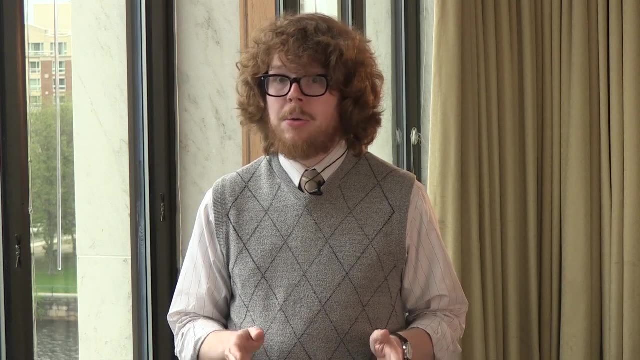 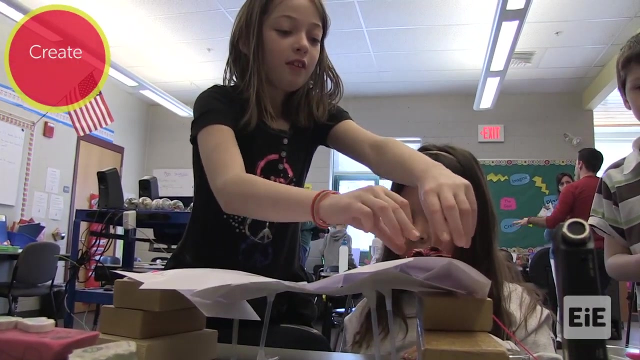 imagined several different ways to solve the problem and come to a consensus about a plan, should they move on to the create step? In this step, students will follow their plan, build and test their technologies. Needless to say, create is usually the most exciting step for students. 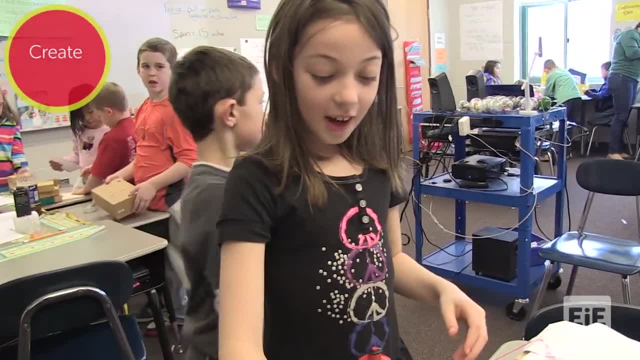 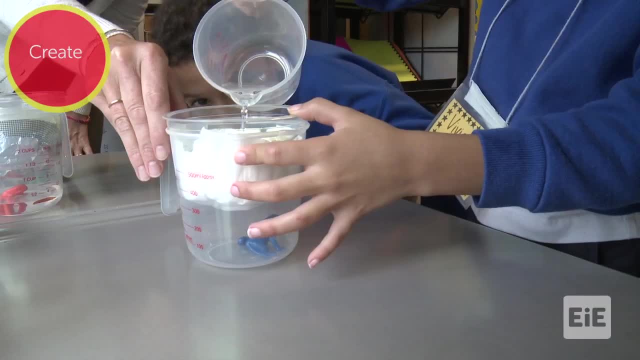 Children are very excited to see their designs in action. Sometimes they work as expected and sometimes they don't. Let's watch a group of fourth graders as they test the model membranes they designed and created When designing a container for a frog. 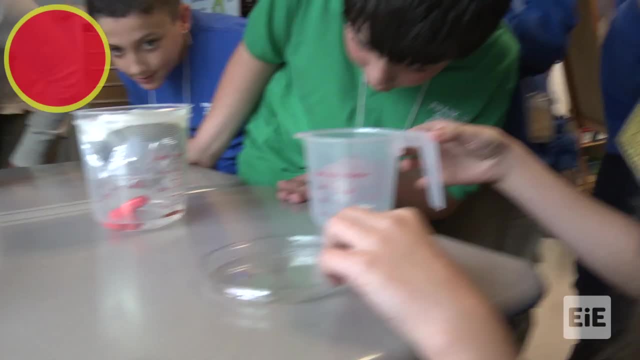 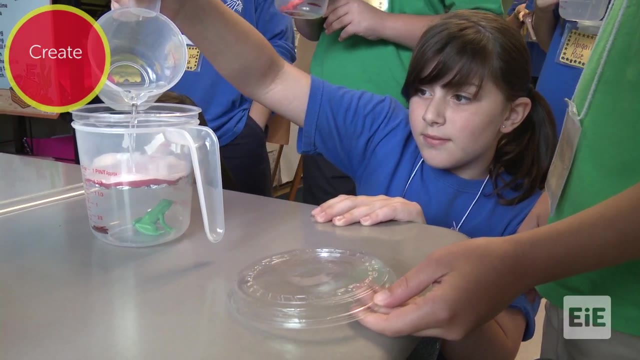 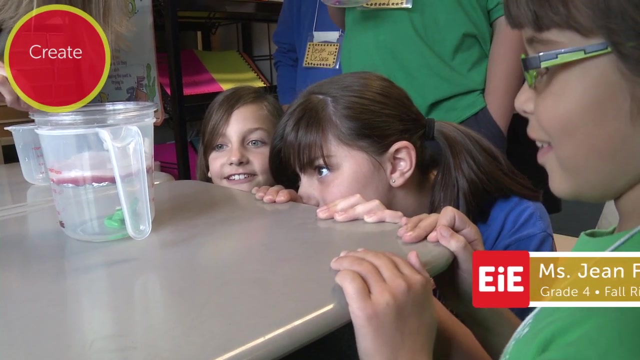 they used various materials to try and reduce the flow of water to a slow drip. What do you think? Fast, Too fast, Oh my god, look, it's already like, yeah, that water's going to be gone, Alright. well, what can you do tomorrow? 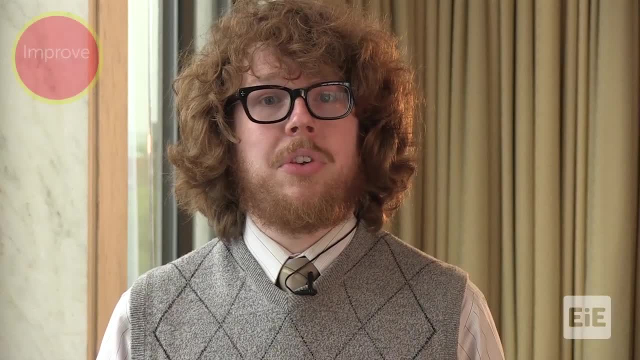 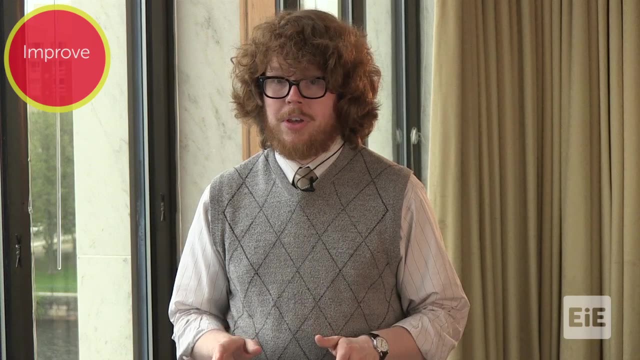 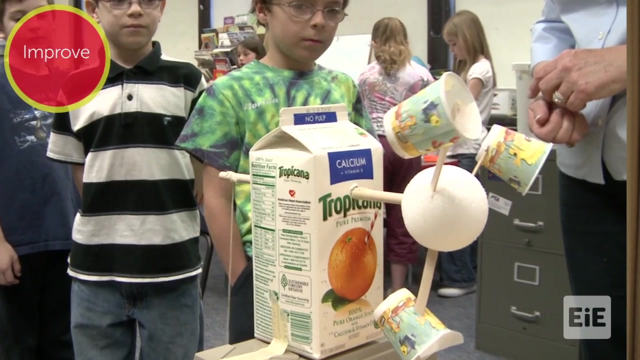 to improve, Put a sponge in it. The improve step is fundamental to the process of engineering. It's important to give your students time to improve their designs. When given the opportunity to improve, students can think critically about what parts of their design are working well. 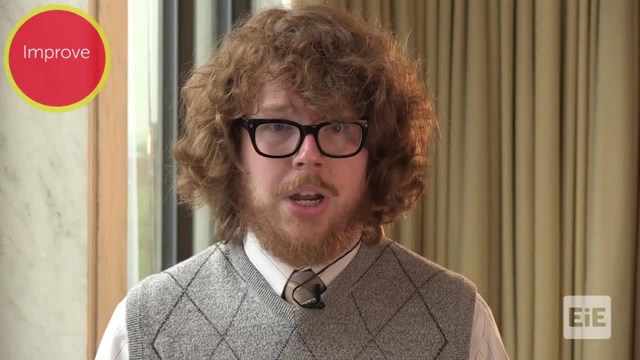 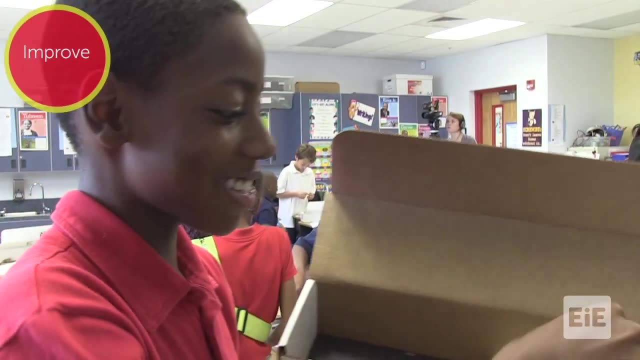 Just as importantly, they can carefully observe what doesn't work. When failure is presented as a learning opportunity and a critical part of engineering, students can think and expect it. In this next clip we see Grace Schofield in the improve step of the engineering design process. 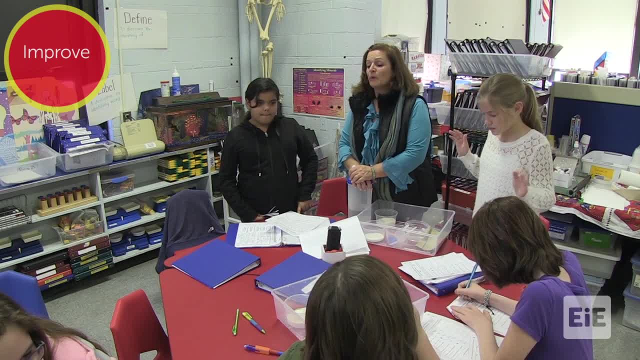 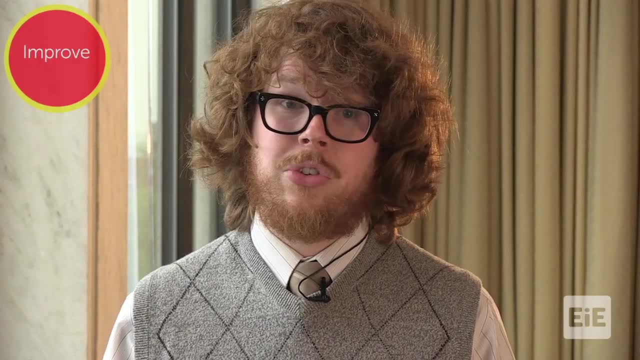 as she leads her fifth grade students through the design of a high quality Play-Doh. Notice how she stresses that the improve step is never complete. Indeed, it's just the beginning of another iteration of the engineering design process. I'm seeing lots of interesting things. 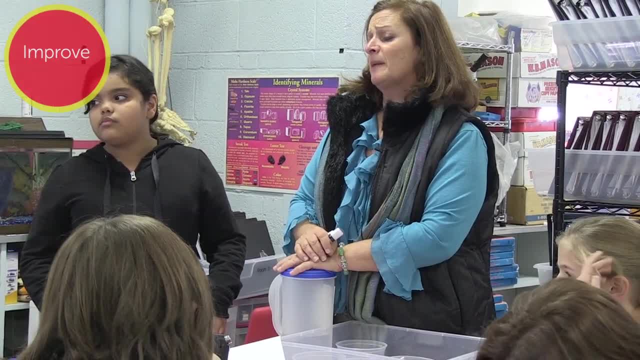 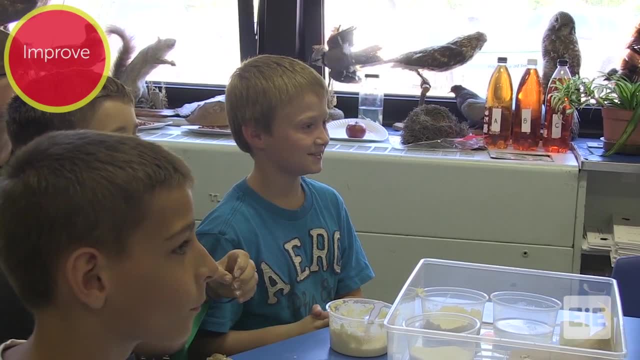 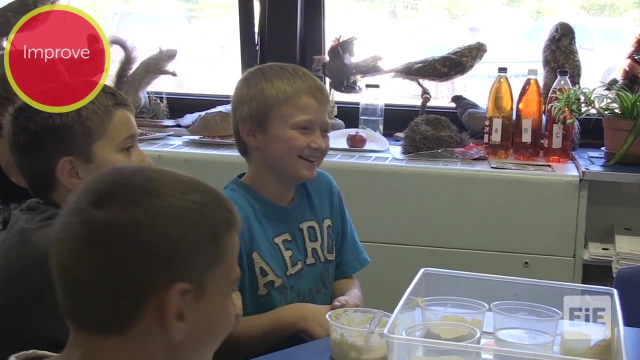 going on. alright, Jordan, tell us what's happening at your table. Oh, we added um, like What? You went ahead, Yeah, And added: Yeah, What step is that? Uh, the improvement. You're gonna improve the improvement. 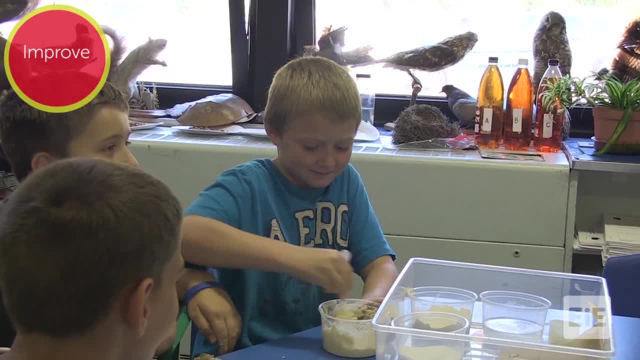 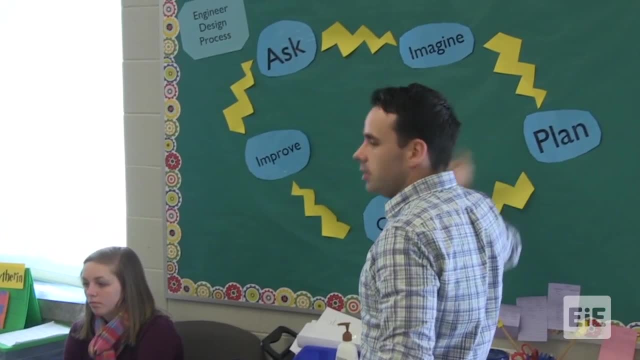 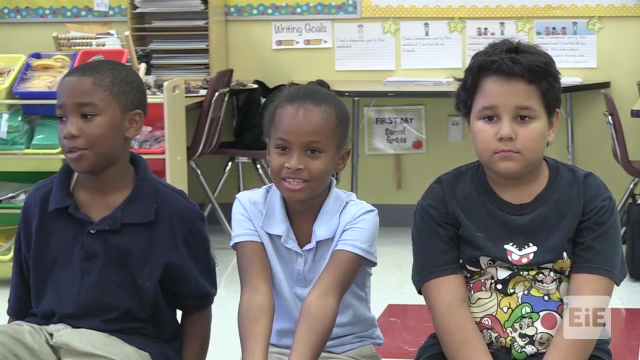 Yeah, Do you see how this is a process? Once you keep doing it, it goes going on and on and on and you're not done, Just like professional engineers on the job. your students may not move sequentially to the next step If you don't do the design process. 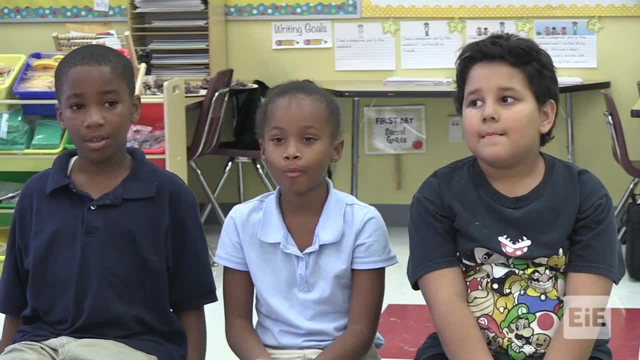 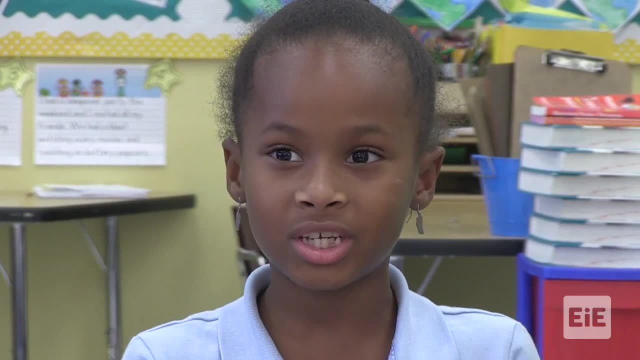 and you want to build something or help with something. you don't know how you're going to make it and you don't know if it's good enough, because you're just gonna build it and you don't know if you need something or if you need to improve something.